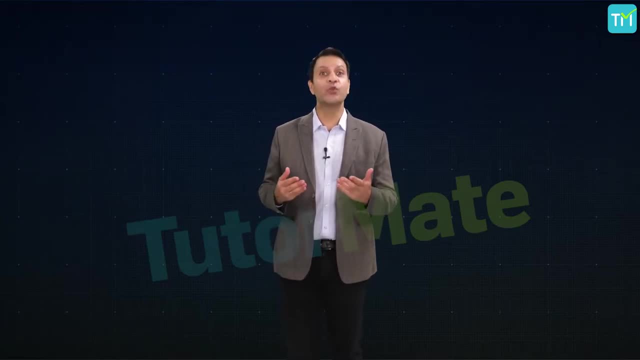 Have you seen a magnifying glass though? Actually, have you touched a magnifying glass? If you have, then I'm sure you know that it doesn't have a plain surface. Instead, its surface is kind of bulging outwards, isn't it? 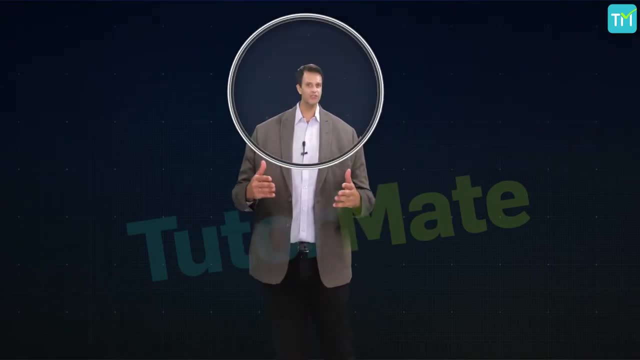 There's a specific name for glasses that have a curved surface, and they're called…. Wait, Are you laughing yet again? Seriously, Why are you laughing this time? Oh dear, I really need to get these five lenses out of my way. 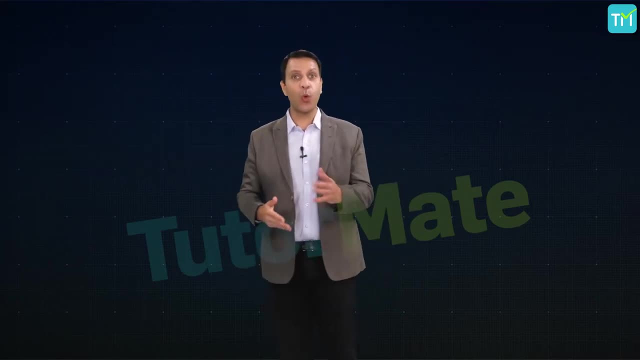 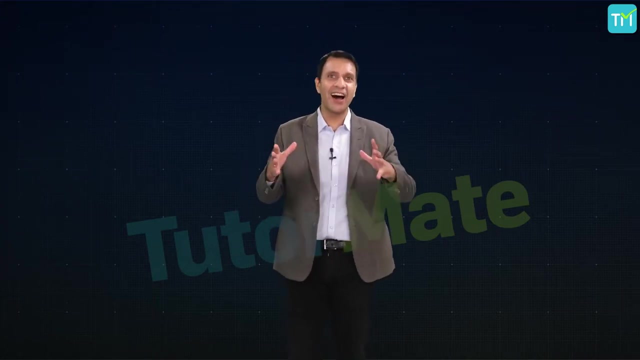 And that's exactly what they're called – lenses, That's right, A glass that has one or both its surfaces as curved outwards or inwards, as a lens. So far, you have laughed at two of my faces that were distorted by lenses. 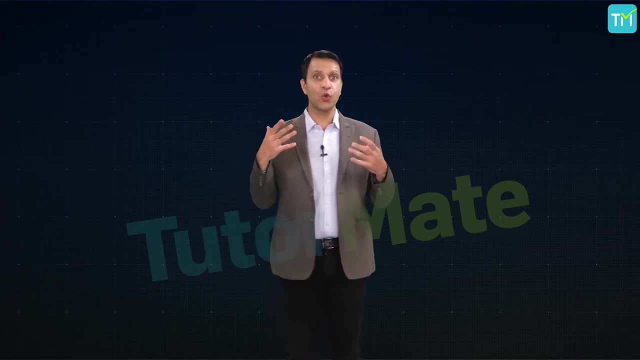 In the first one, if you observe, my features looked bigger than they really are, And that was achieved using a lens that was bulging outwards, which is known as a convex lens. The second: you must have seen that my features looked smaller than usual, which was achieved. 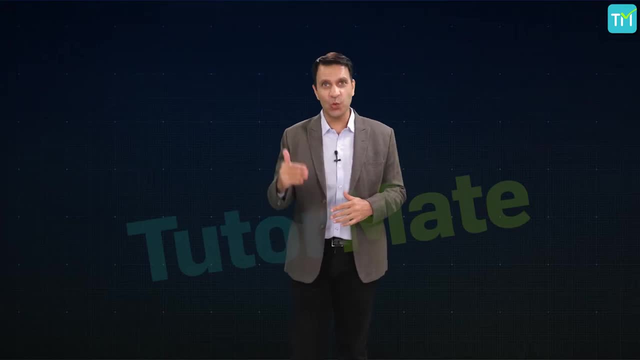 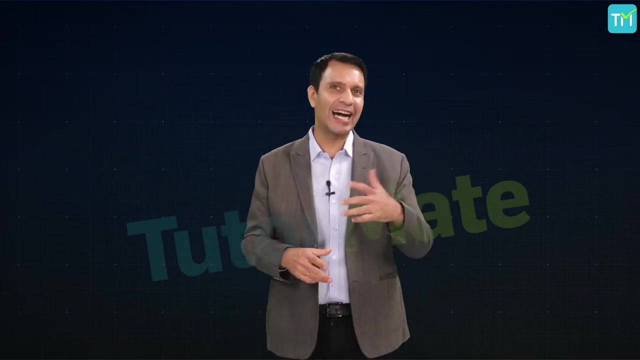 using a lens that curves inwards and is known as a concave lens. Now let's study more about these lenses and see why they distorted my lovely face like that. Before that, let's do a quick recap of the definition of a lens. According to the definition, a transparent. 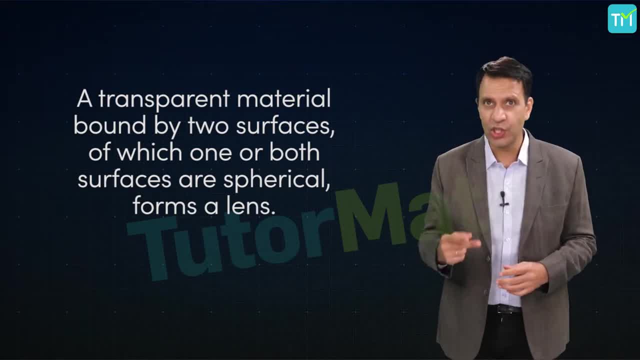 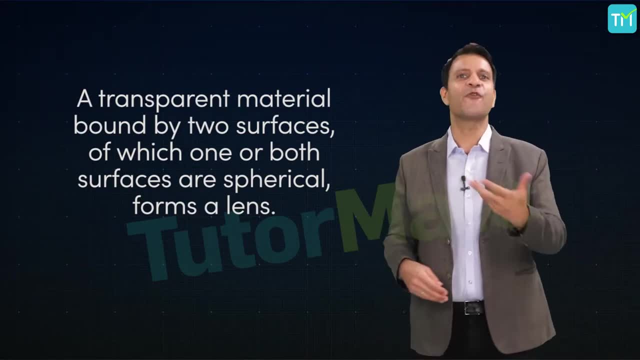 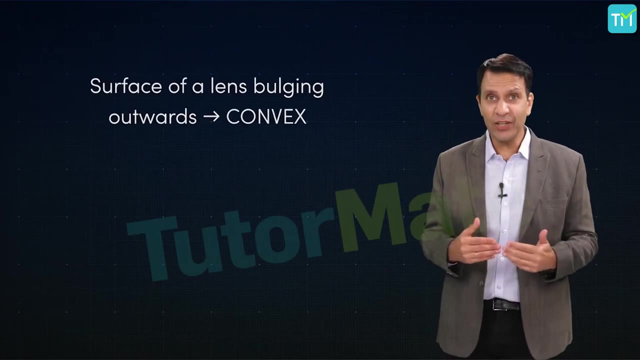 material bound by two surfaces, of which one or both surfaces are spherical, for which one forms a lens. So let's try different combinations of these surfaces and see the kind of lens that we get. But remember one thing: Whenever the surface bulges outwards, 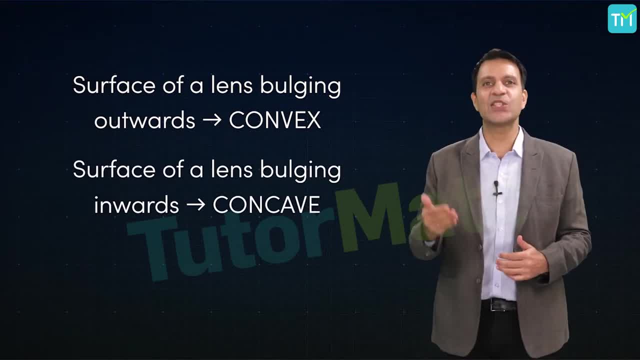 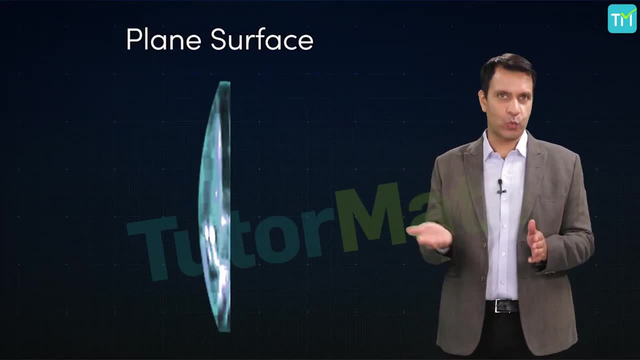 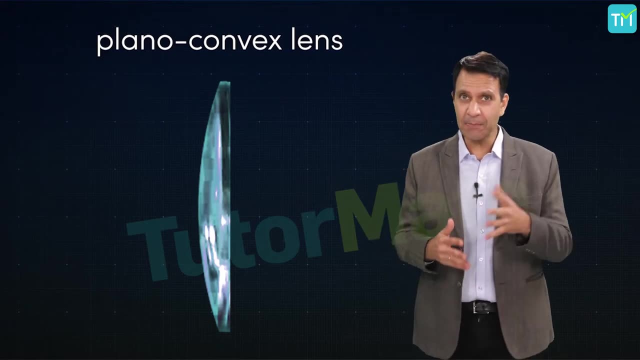 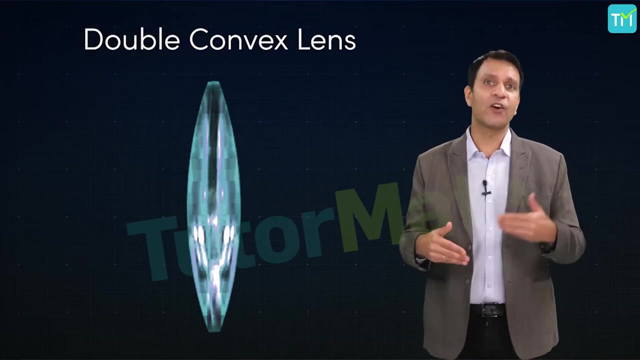 it's convex and whenever it curves inwards it's concave. Let's say we have one plane surface and the other surface bulging outwards. This type of lens is known as a plano-convex lens. At the same time, if we have both the surfaces bulging outwards, the lens is known as a double 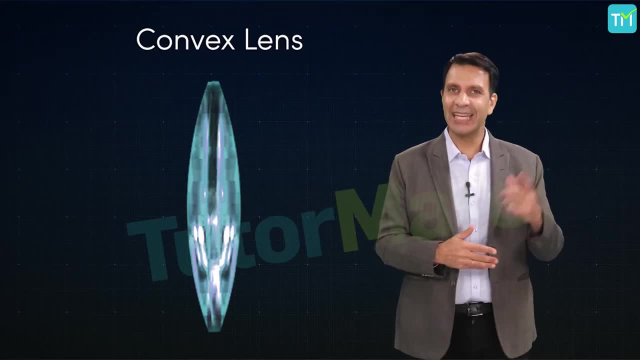 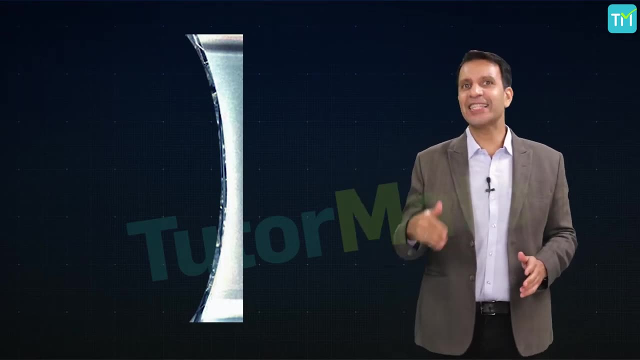 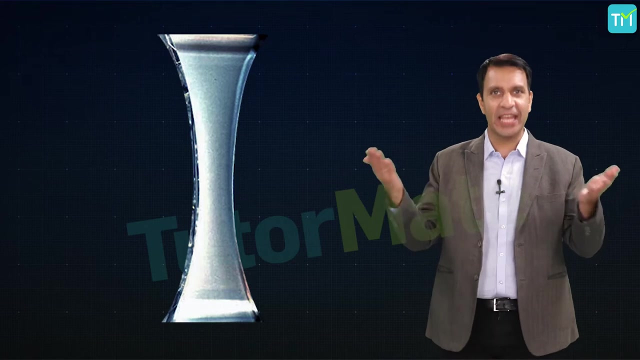 convex lens or simply convex lens. Next, if we have one surface as plane and the other curving inwards, then the lens would be a plano-concave lens, And when both the surfaces are curving inwards, the lens would 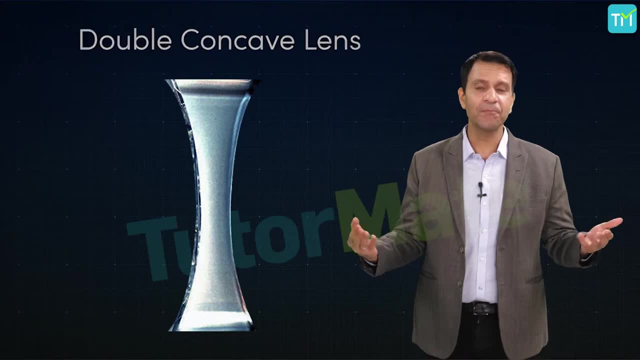 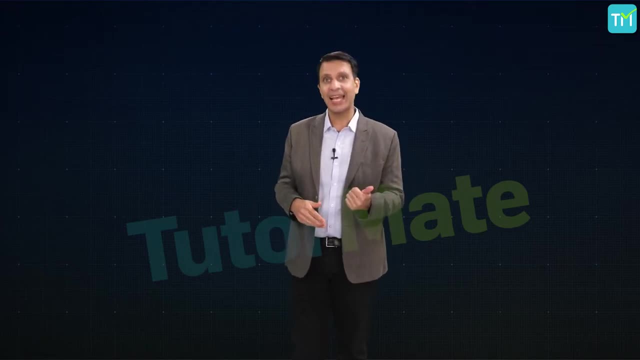 be a double concave lens or simply convex lens. We are going to be studying how refraction occurs in the double convex and double concave lenses, So we'll only refer to them as convex and concave lenses respectively. okay, Great. 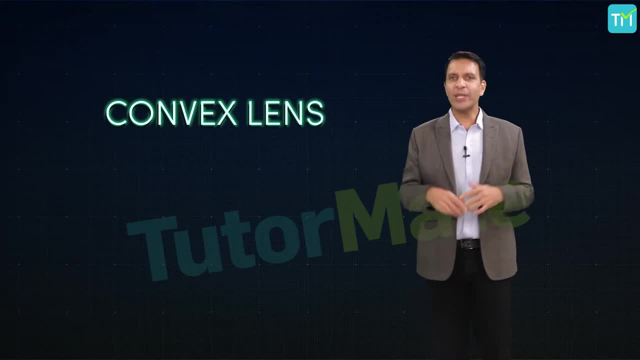 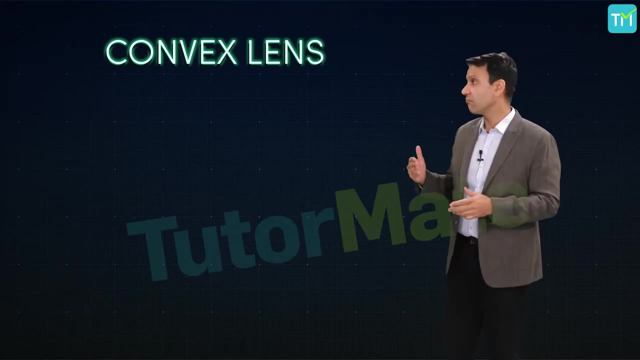 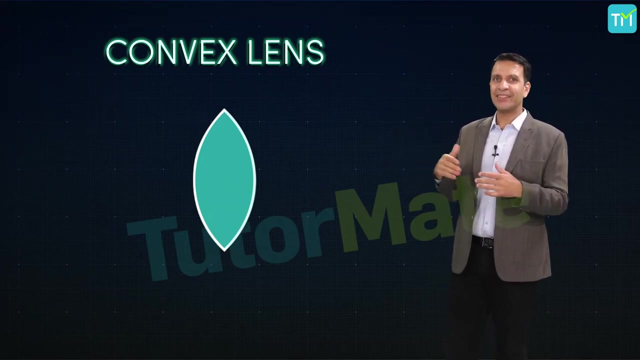 Let's consider the convex lens first. We can actually visualize the convex lens to be formed by the parts of two spheres like this: There are two centers of curvature of one convex lens, and these two are represented by C1 and C2, as you can see here. 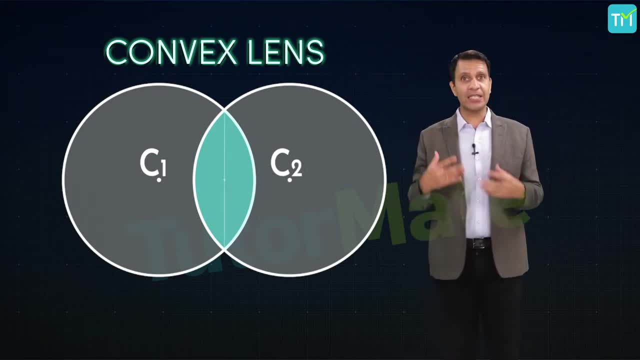 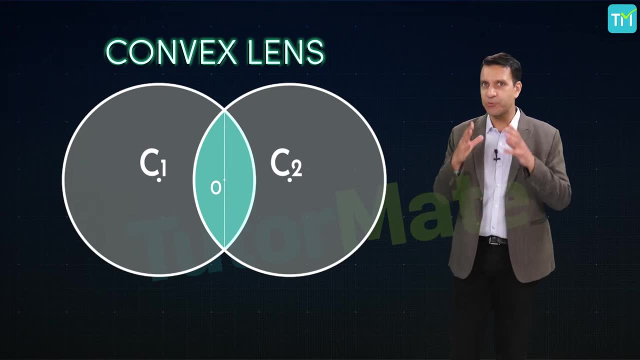 But the lens also has an optical center which lies in the middle of it. It is denoted by the letter O, And the special property of the optical center is that any ray of light passing through it will not undergo refraction. So let's consider the convex lens. So let's consider the convex lens, And the special property of the optical center is that any ray of light passing through it will not undergo refraction. This is called a linear fijation, which means that any aberration will follow after refraction. 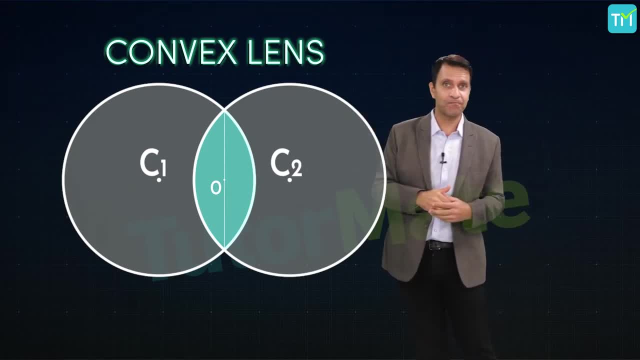 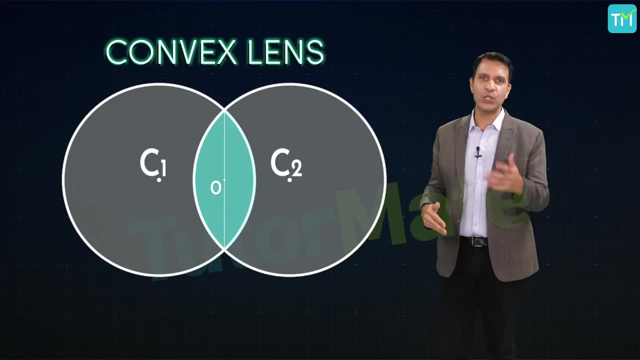 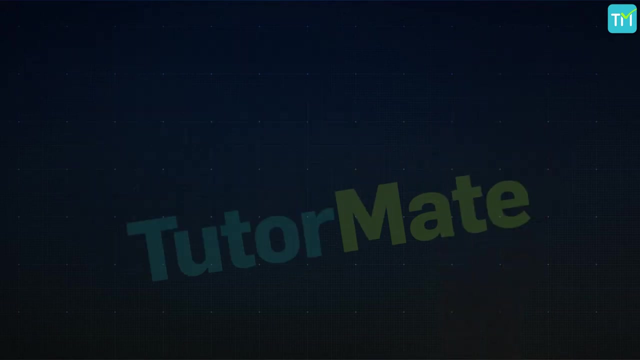 We can call this a linear deviation, and we'll travel in a straight line through it. The principal axis is also perpendicular to both the faces of the lens at the points where it intersects them. Next, a convex lens is also known as a diverging lens. 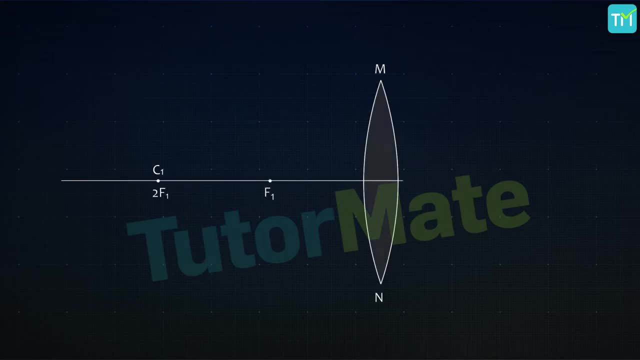 It is nowhere, by any chance, known, unless we look at beleurs in the blue. Absolutely, This box, wrapped curve on the middle. Can you guess why? That's because it diverges the rays that pass through it. Let's say we have a beam of light passing through the lens, where the beam 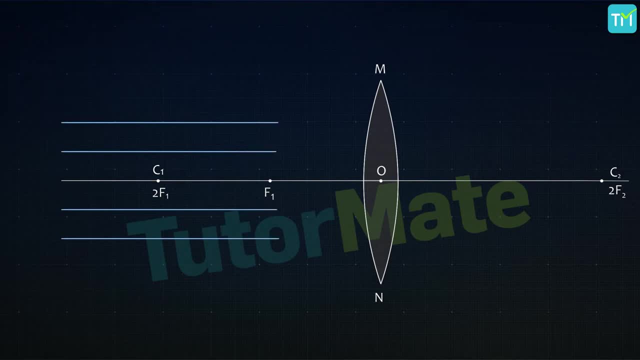 of light has light rays that are parallel to each other and are also parallel to the principal axis. When all these rays pass through the lens, they undergo refraction that is governed by the laws of refraction and they bend towards each other. Finally, they all converge and meet at the same point. on 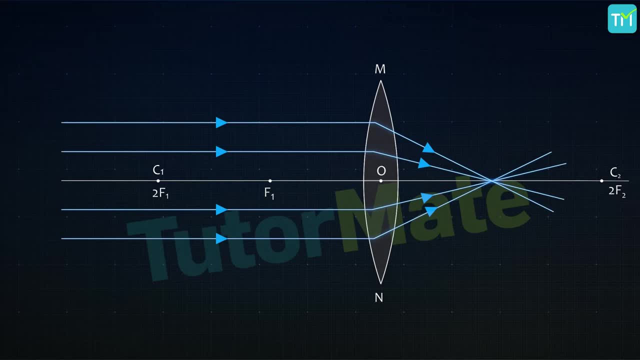 the other side of the lens. This point, where all the rays meet after refraction, lies on the principal axis of the lens and is known as the principal focus, denoted by the letter F. At the same time, if we had instead made the beam of light fall on the right face of the lens, then the rays would have. 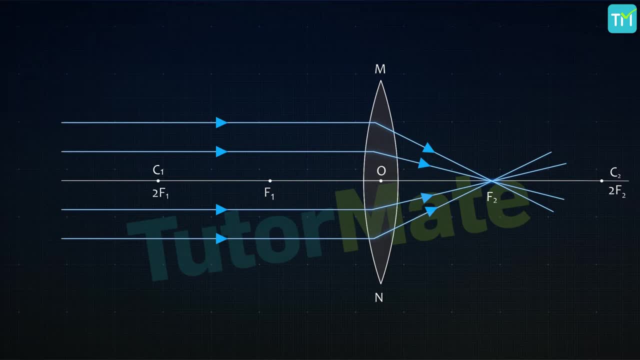 converged to a point- the point on the right face of the lens- then the rays would have converged to a point on the left side of the lens, which also lies on the principal axis. Even this point is known as the principal focus. This means that the lens has two foci, which are at 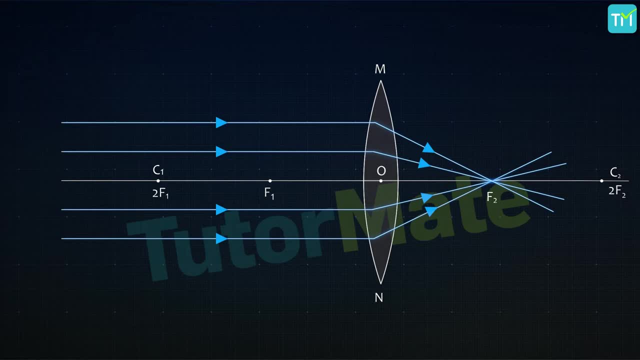 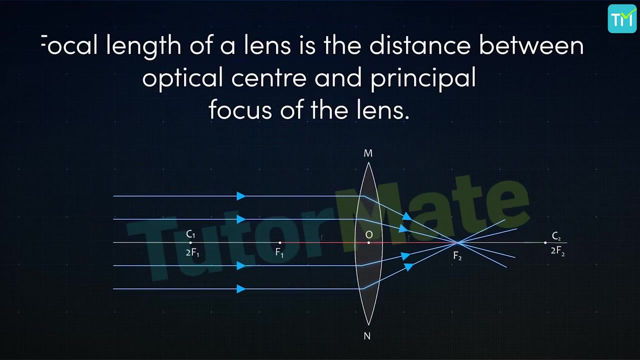 equal distances from the optical center, and they are denoted by f1 and f2, and the distances OF1 and OF2, which are equal to each other, form the focal length of the lens, denoted by the small letter f. Therefore, by definition, the focal length of a lens is the distance between the optical center and the. 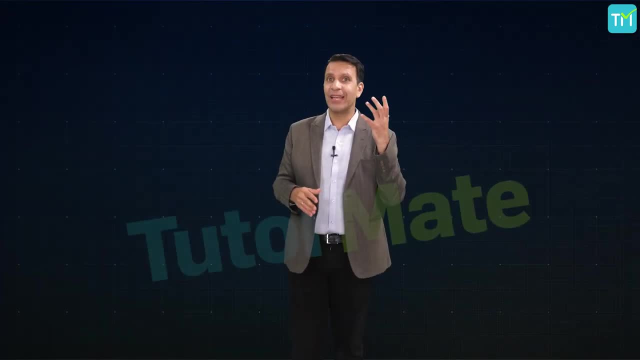 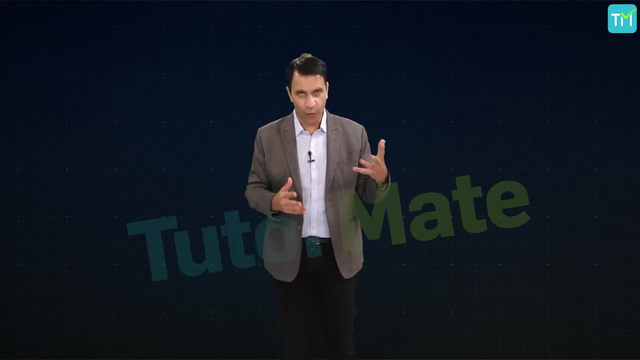 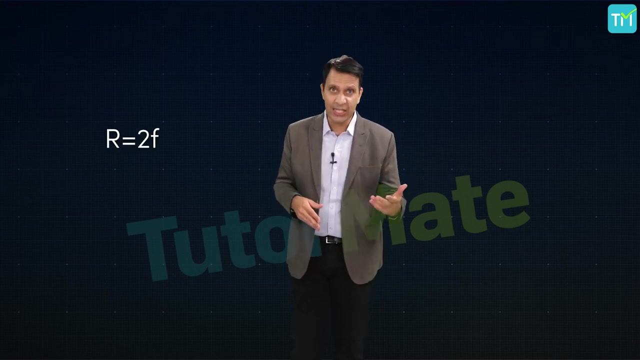 principal focus of the lens. Also, the focal length of a lens is half of the radius of the curvature of the lens. Therefore, if r is the radius of the curvature we get, r is equal to twice of f or 2f. Do you remember that one experiment we did with the concave? 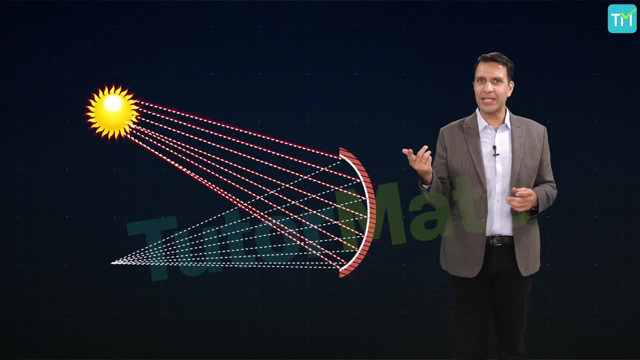 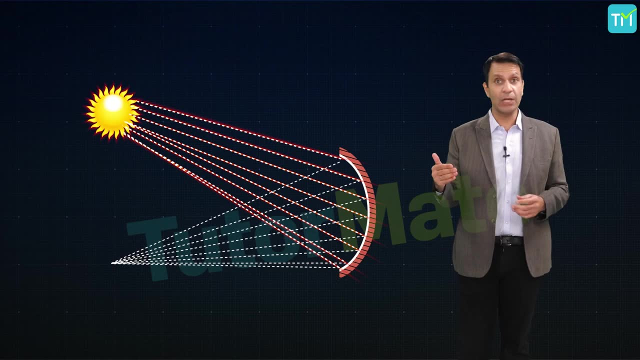 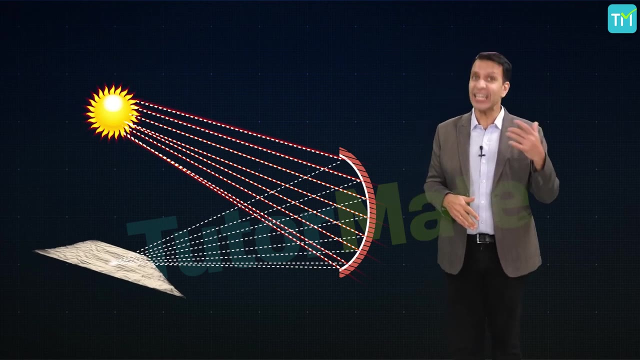 mirror and the Sun. Yes, the one where we obtained the image of the Sun at the focus of the mirror and ended up burning a hole in the paper. So let's do that again, except this time we'll use a magnifying lens, which is a convex lens, instead of a concave mirror. So we'll 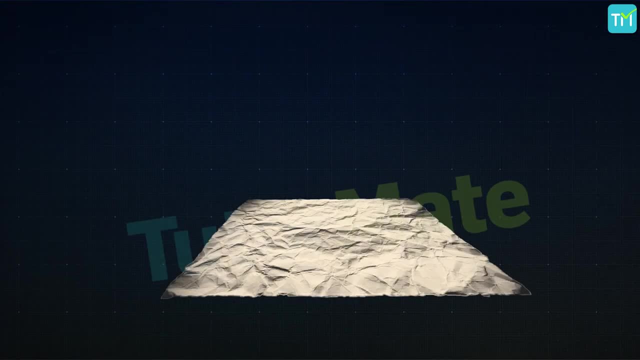 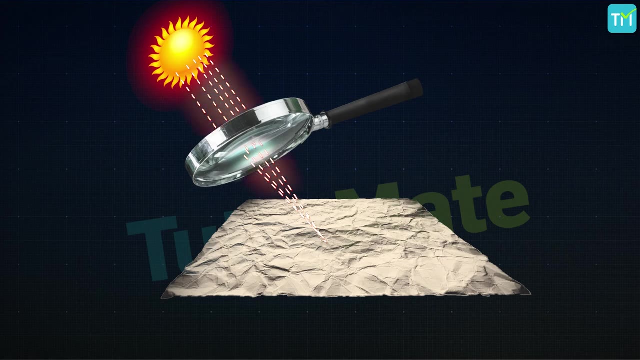 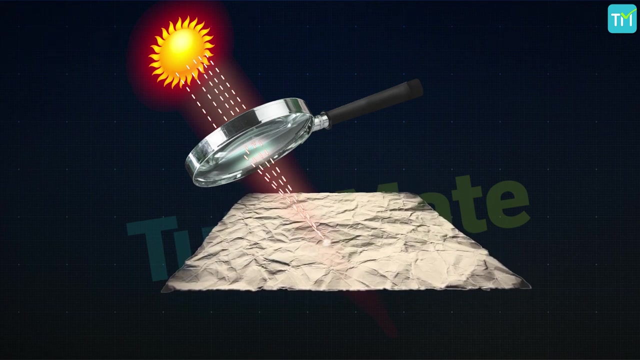 take a sheet of paper and hold it below the magnifying lens, Then we'll go out in the Sun and try to focus the Sun's rays on a single bright spot on the paper by moving the paper back and forth Now, since we have already done a similar,